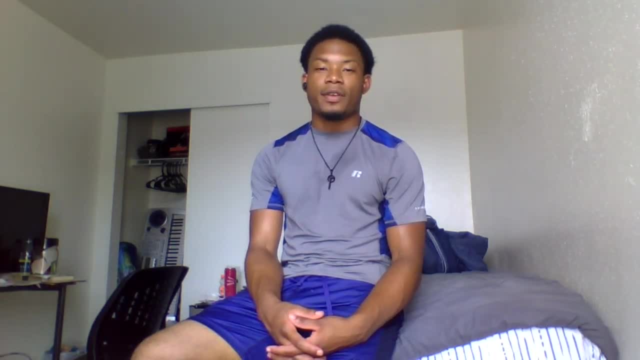 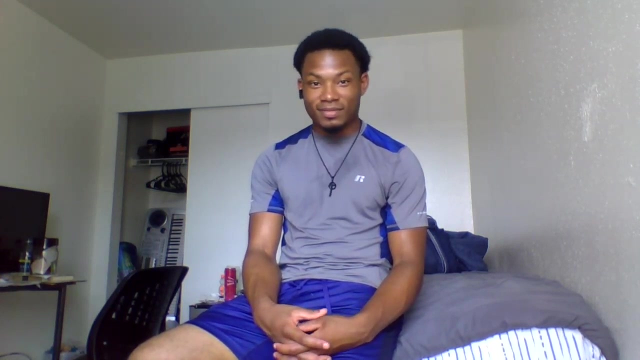 You're going to run across a lot of people who are very good at stuff and we, as musicians, we're hard on ourselves And you may get frustrated, You may get tired out. It's okay, Take yourself a break. okay, This stuff it's not easy, all right. 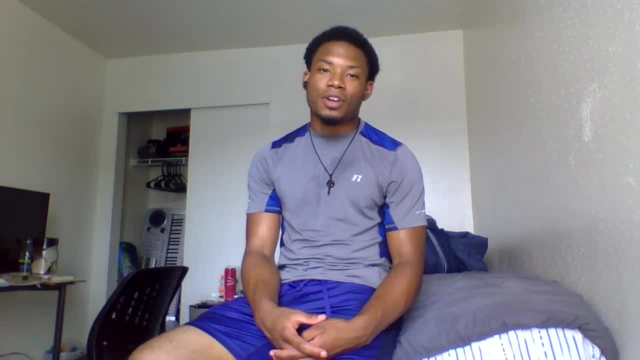 I also wanted to make this video because I wanted to encourage y'all. I want to encourage all my music education people out there And if you're going in, this is your senior year of high school, you can say you want to do music education. So the essential things of 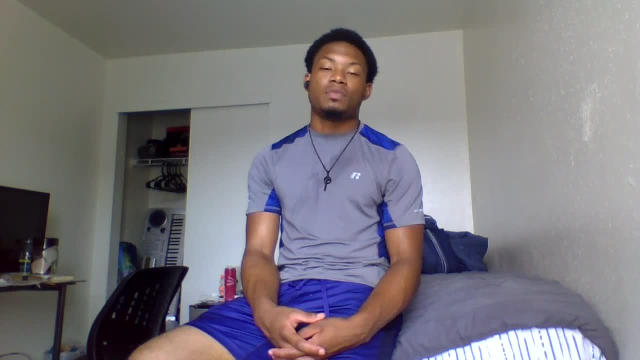 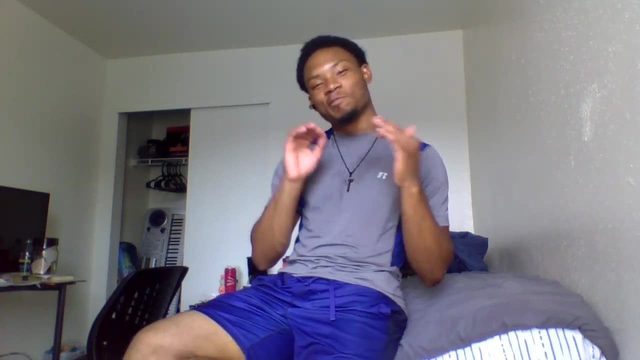 music education you have to learn when you get to college is music theory, music history, aural skills. I'm not good at that either. That needs a little bit of work, but I'm working on it, I am. I'm not going to give up. I'm not. 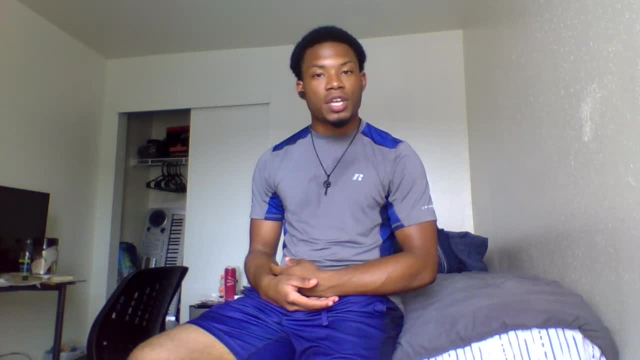 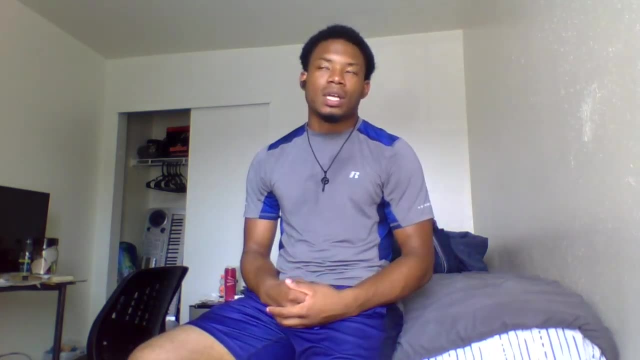 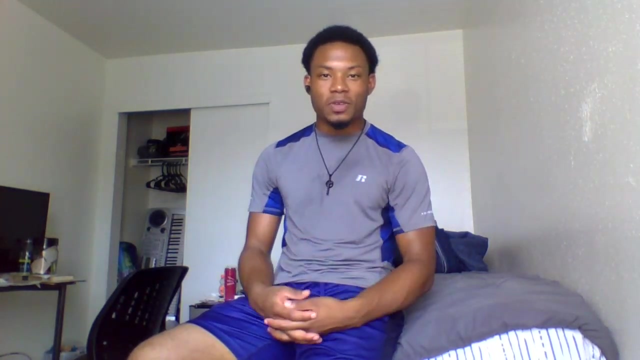 There's that You have your higher education classes. You have some of your other education classes that work towards your certification. when you begin to step into teacher candidacy, You have your- my favorite class is your instrumental methods classes, where you actually play different instruments and learn how to teach them and strategize in teaching and 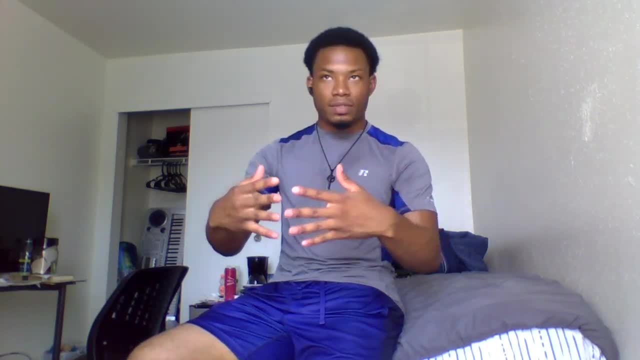 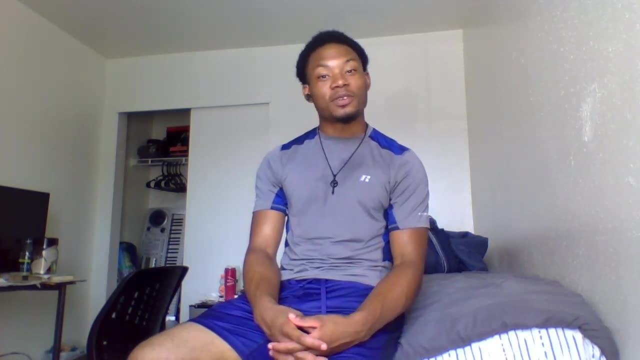 basically learning in more of a pedagogical way of teaching and how the instrument is to be played And what you probably will end up having to deal with whenever you begin your first day of your first year of teaching, And so you'll learn stuff like that. 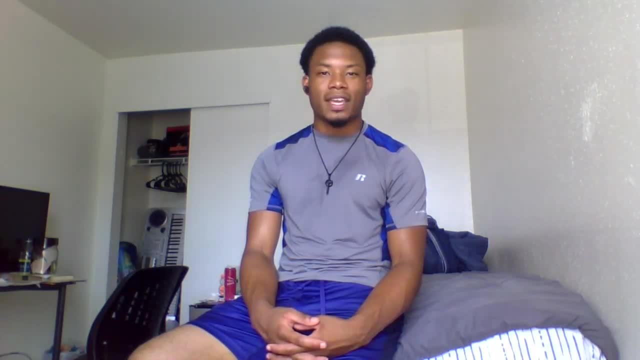 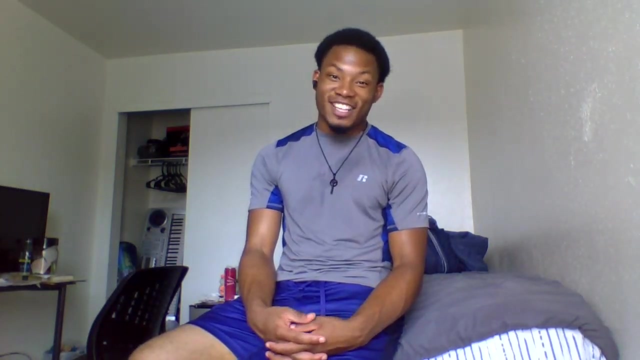 You'll also get to know a lot of music organizations like KK, Psy, SAI and what's another one- TBS. Those are really great organizations. as well as I'm U Alpha, Y'all those guys can sing. Those guys can sing. 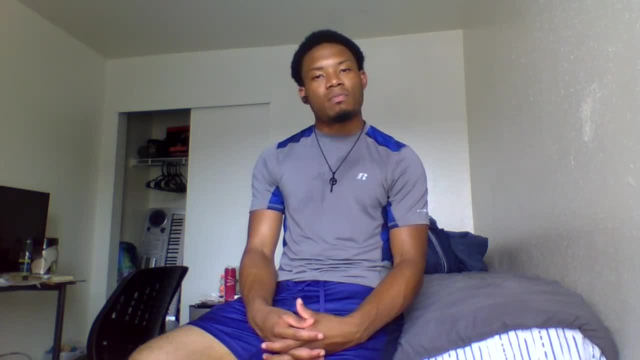 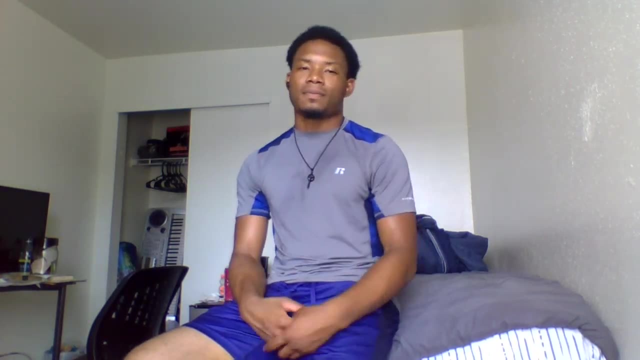 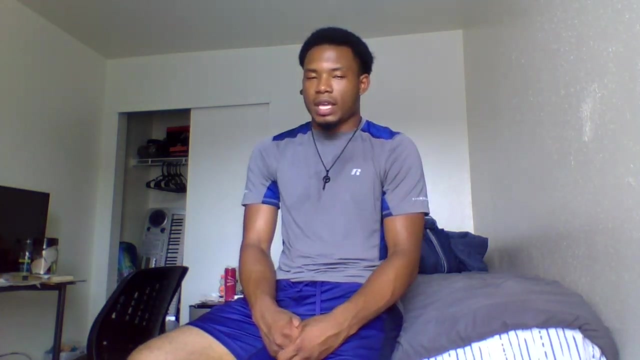 They're awesome. So you get to meet many of the people in the music world. There's a lot of them. But yeah, back to music education. So you're probably thinking, okay, what there's so much? why do I have to know all of this? 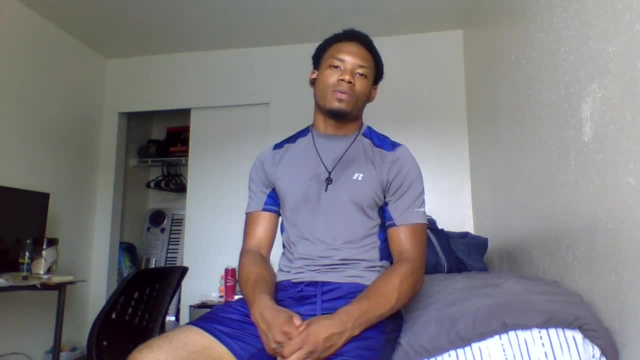 Y'all I thought the same thing: Why do I need to know music theory? Why do I need to know music history? And it took me awhile But really began to see that okay, because at first i was like i'm not gonna, i'm not gonna use this. 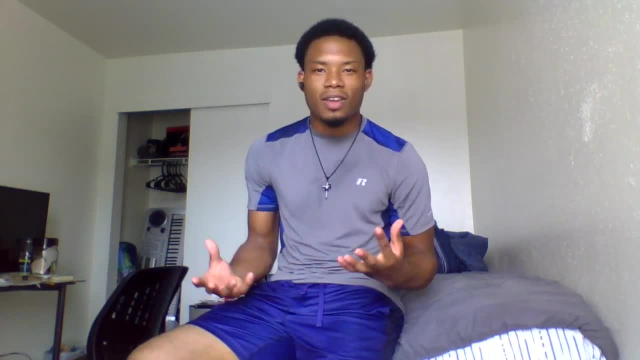 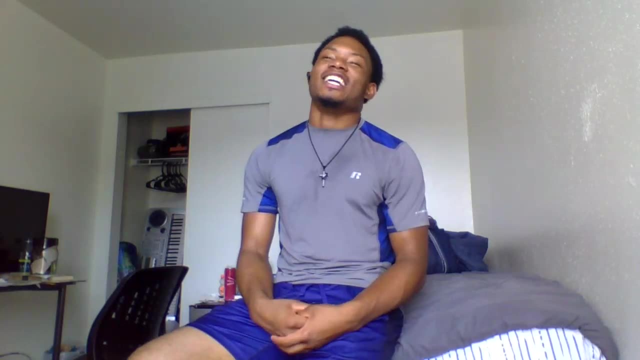 like none of my band directors. they asked me. i asked them, like, do y'all even use this stuff? and they would tell me, no, you don't. so i'm like what's the point of me learning? so i realize it is important because i saw it as a part of my education as a music person, as a as. 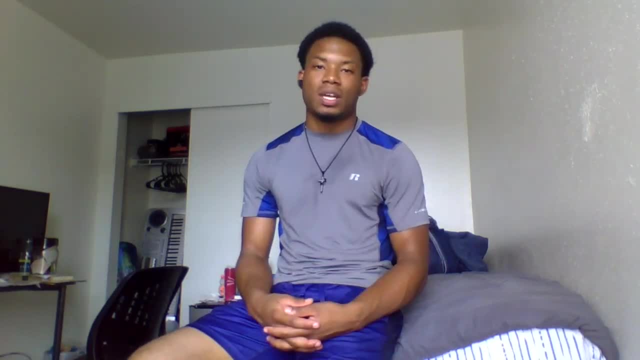 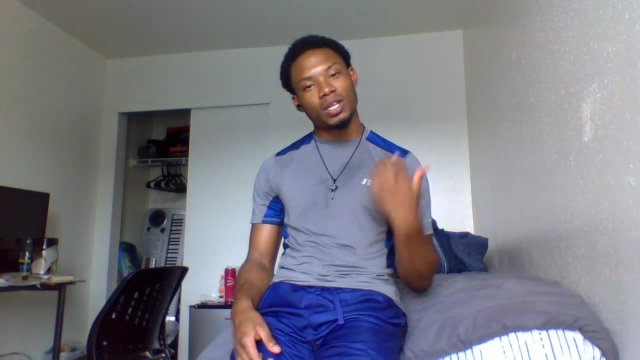 a intellectual, as a music intellect, to understand you know how this and that works and um, you're gonna come across a lot of stuff. and oh, piano class. yeah, i forgot that, one do not forget. you're gonna have to take piano lessons along with your, your um, your main instrument. you can take lessons. 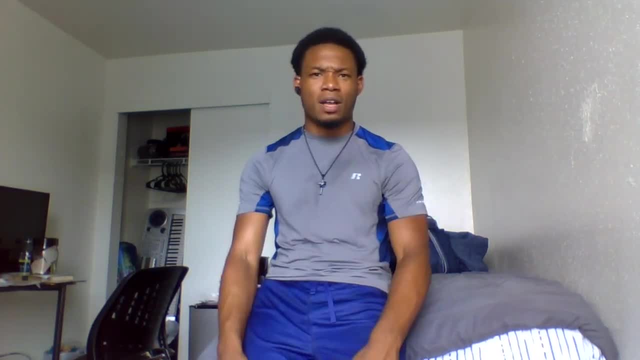 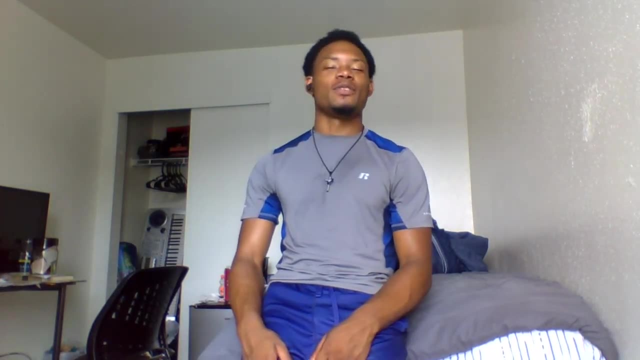 on that too, as well as juries. i think some of y'all may call it juries, some of y'all may call it the end of the world, but uh, if you're a music major, you know what i'm talking about. but um, yeah, um, i forgot i was going. 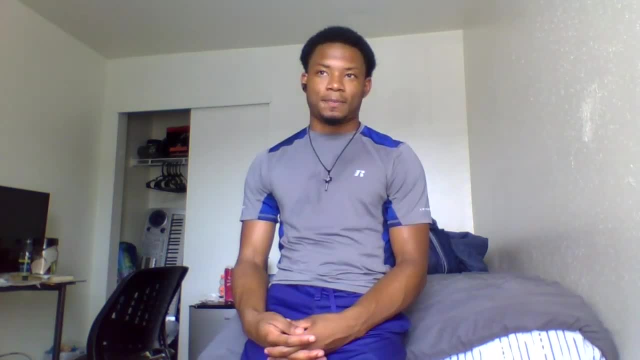 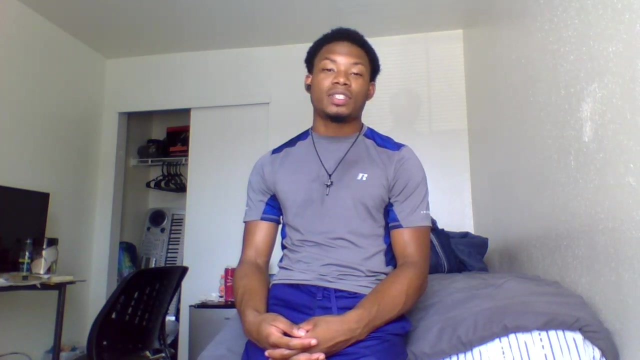 with that. but yeah, so you have all these essential things of music education that you will, uh, you'll get to know and you'll learn and you will struggle. if it comes easy, it's great. if it doesn't work hard for it, all right. you may walk out of class with tears, you may. 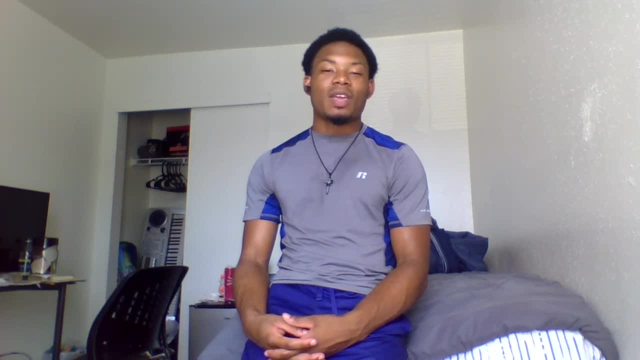 you, you, you may even doubt yourself, you may even ask yourself: you know, is this even what i want to do? and you know, that's fine if it is, if that's the questions you ask yourself, it's cool. you know, be honest. if you, if you want to work towards, you work towards. if you feel like you can do something. 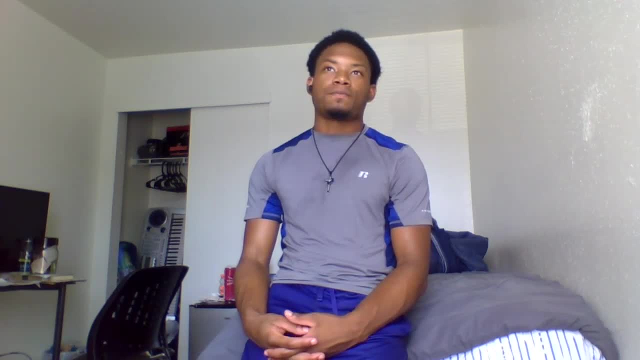 do something else. you do something else, but push yourself. okay, music education is not just okay, a show-off kind of thing. okay, this is a degree that i've come to understand, that this is for you, but it's not just for you, it's for the future, it's for our future musicians. 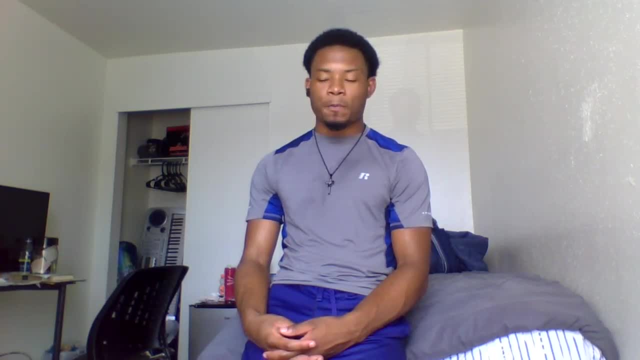 and a lot of you who are in band now. you know you have that band director right now. they may get on your nerves, but when you are around the third year of college you will remember them and everything they've taught you about life, about music, about how to carry yourself. you know the professional. 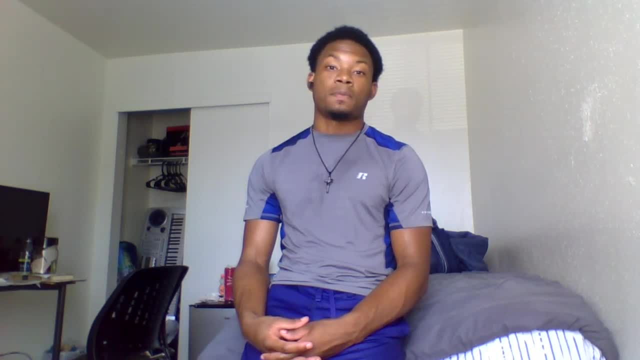 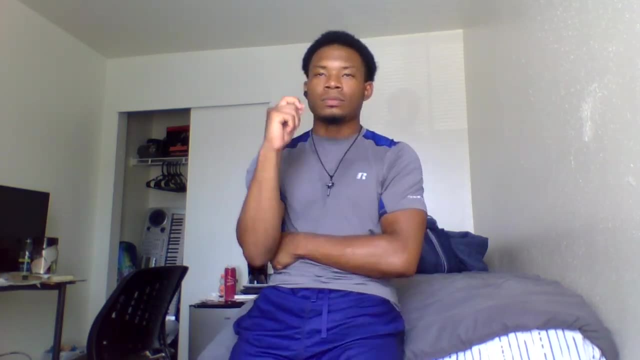 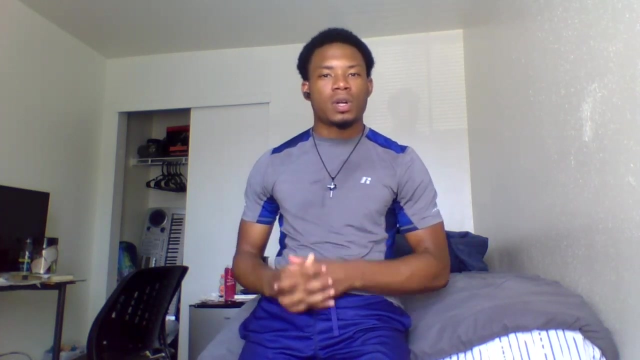 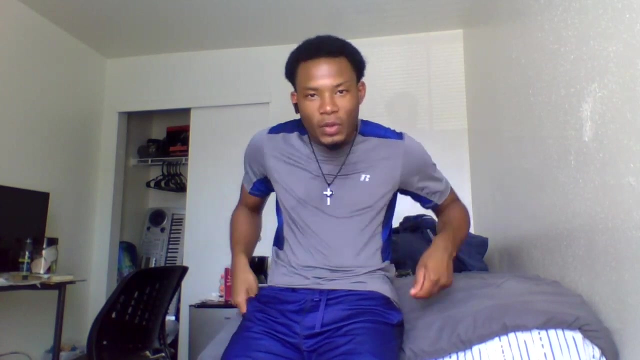 manner and you're going to miss that, you're going to miss them and music education in itself. i, i've come to realize and see that it is to help build our future as a culture. you know music as a music in general and you know in itself, because music, you know we, as music people, we, we love it, we, we, we can't, we can't. 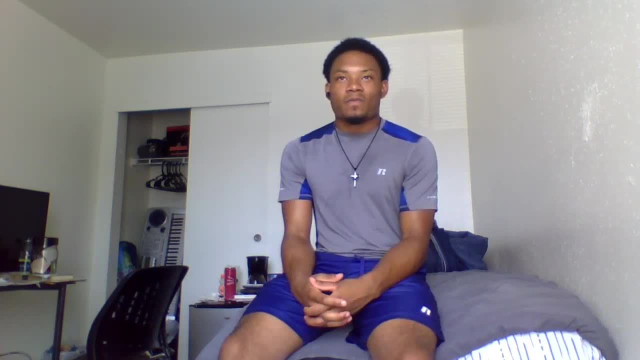 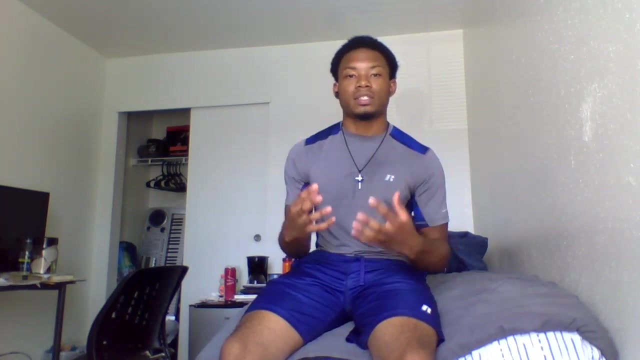 we can't. we just love it a lot and look at that as your, you know, as your goal. you know the reason why i said it is because this is all for the future, this is all for the kids, this is also for you to express how, how awesome music is, because these little kids, they don't know. so you, 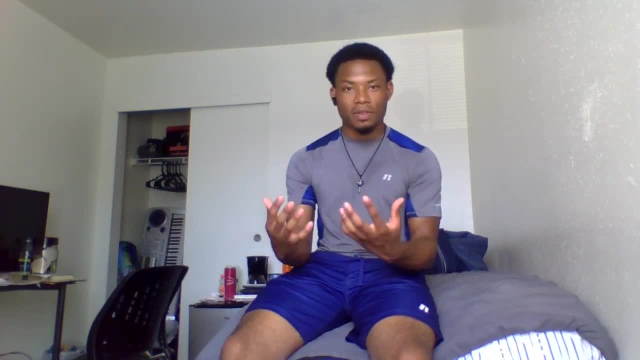 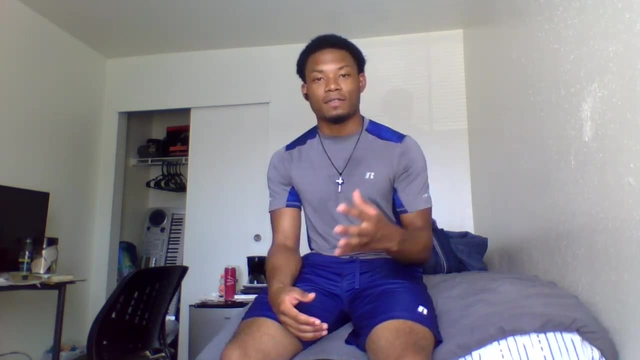 have to, like, give them and help, nourish that idea and build it with them. you know, and so you know, with that being said, you have to give them, and give them that love of music. all right, because it's not just gonna, you know, help them, then it's going to be, you know, it's going to be, you know it's. 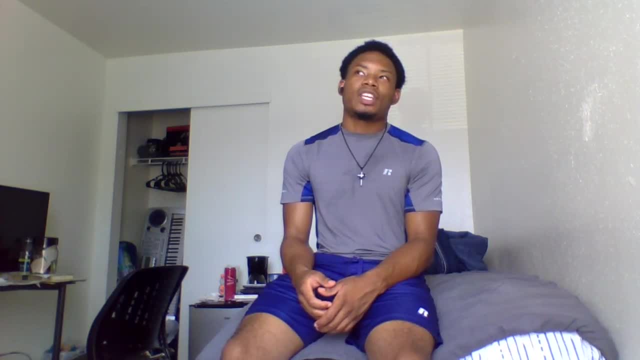 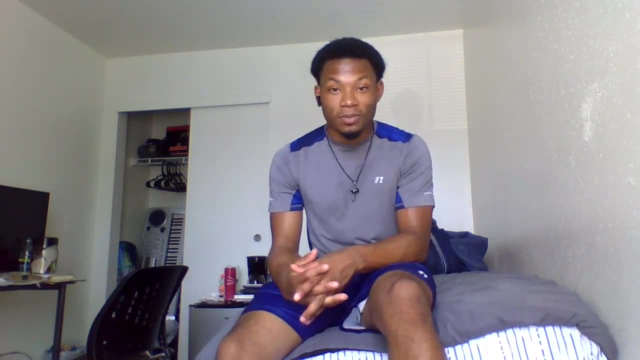 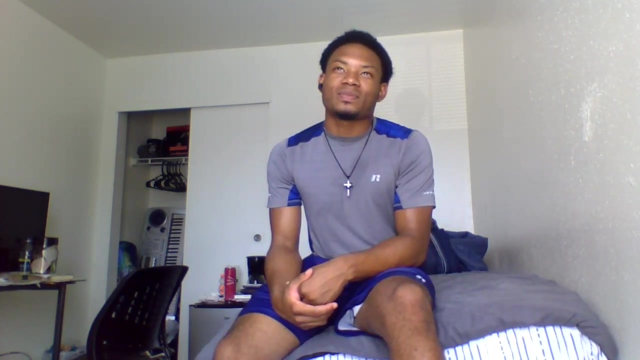 going to help in the future and music education helps build that and it establishes that and a lot of these kids they need that, they really do. y'all, our generation right now. i'm a 1996 kid, i'm a 90s person, i'm a 96 baby and my generation, compared to the generation now, is totally different. 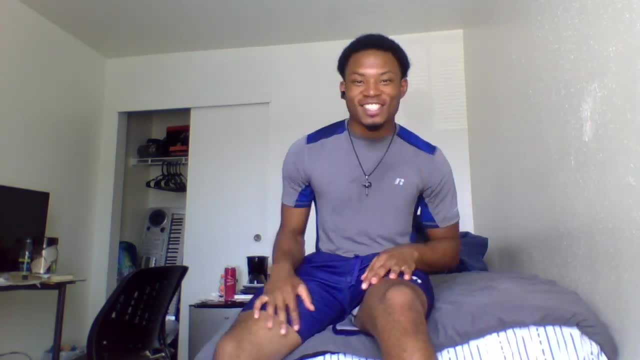 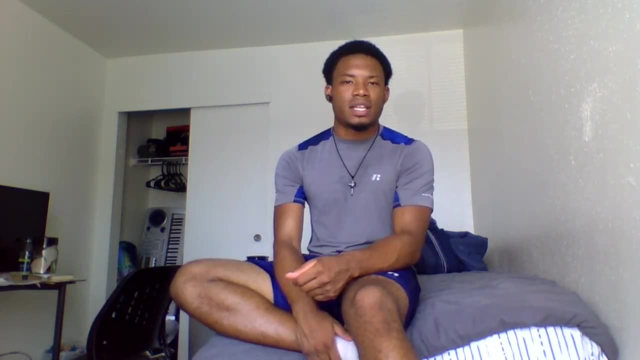 and although we're kind of up to date with the technology, of course, but you know, in general kids in this generation, they need music also and as music educators or future music educators, we need to push that all right um, and that involves with us learning and being the best that we can be, you know. 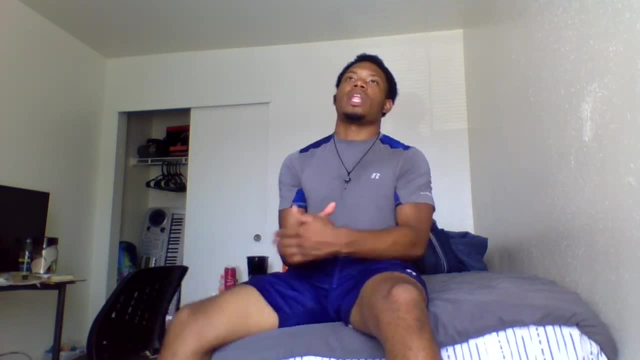 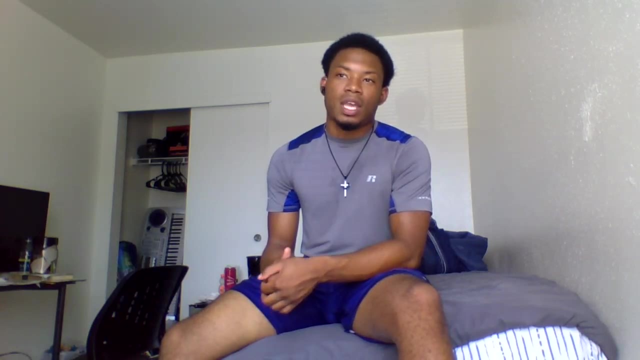 whether you're good at it or you're bad at it, there's always something- and i realize this- there's always something that you will pull and pick from and it'll become your strength and it'll be. and you may think you've spoken. all right, you've been there and all right, you have fun there. you're a pro, you're. 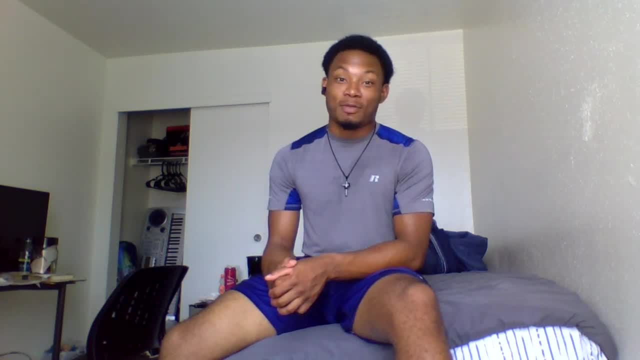 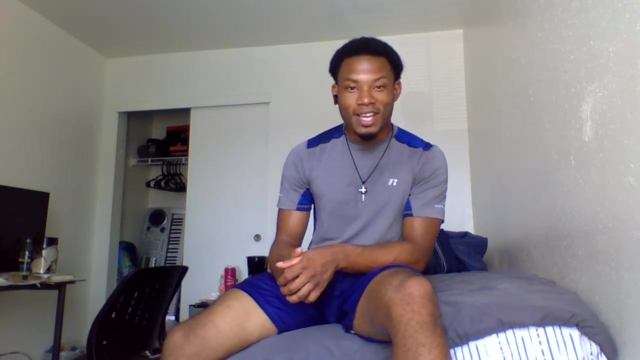 always gonna be great and you're gonna do it because, as musicians, again, we are hard on ourselves and we're perfectionist. yes, we're perfections, and i hate that. i really do. i can't stand it, but it's true. but i think that we get in the way of it because a lot of us, we're also. 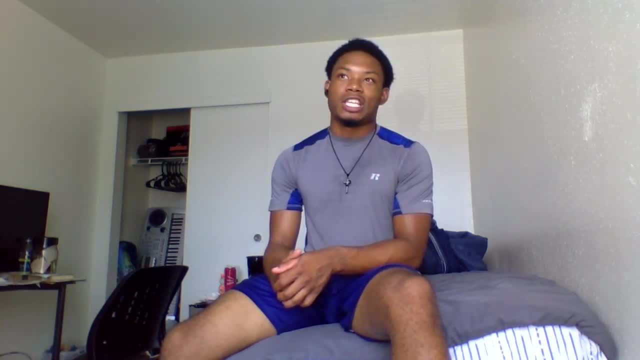 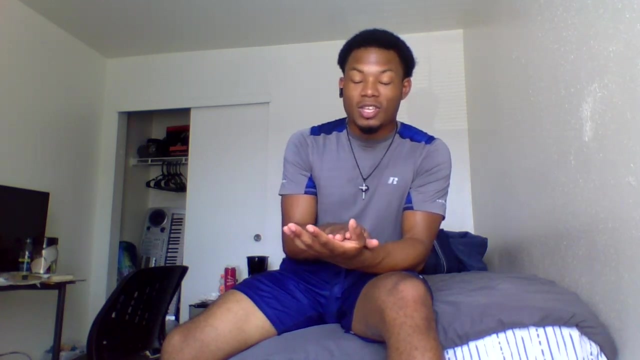 show-offy with some stuff. oh, i can do this and i can do that and all that. yeah, that's nice. but the strengths as well as your weaknesses, to be able to teach that one kid you know, to be able to establish, you know, to help that kid establish a great basic knowledge of music better yet, can you? 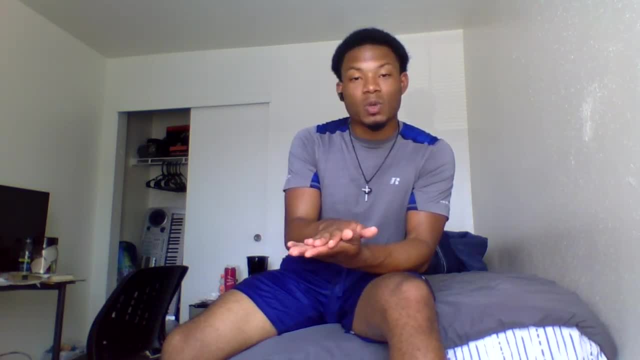 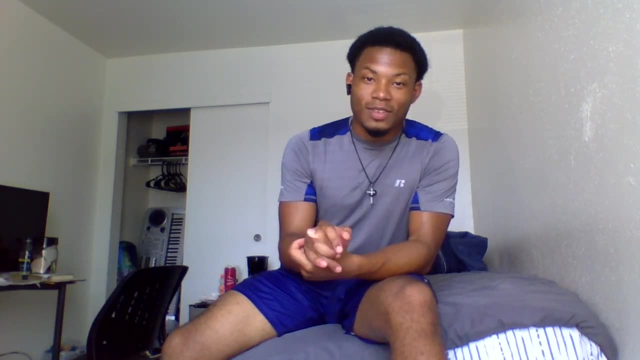 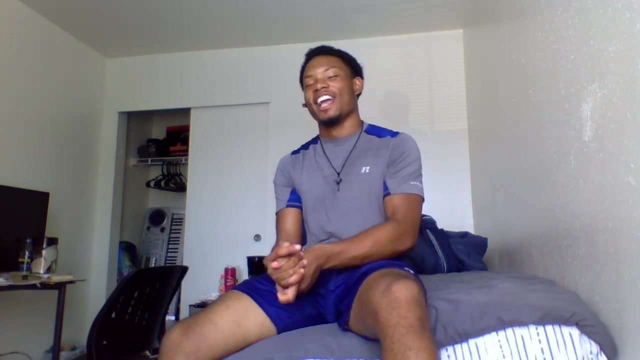 help that kid and encourage that kid to either one day pursue music. you pursue music even more. you know that's important, even though we all know you can play melodic and harmonic scales over and over. uh, with your eyes closed and with your hands behind your back, not even care which string you're. 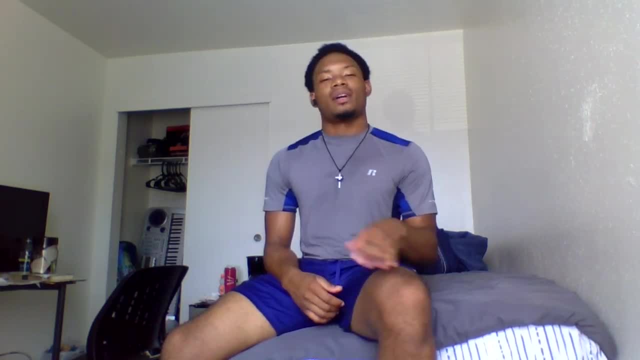 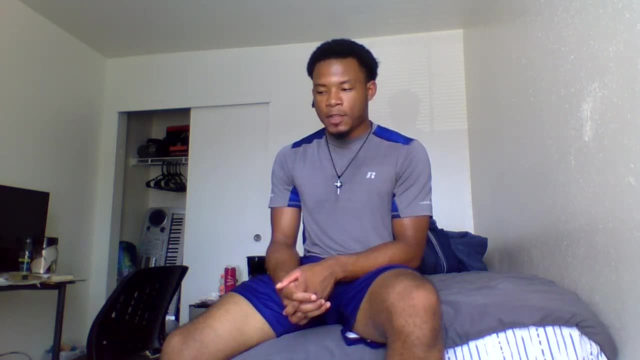 on, but um, but yeah, you know, music education, i see, is this, this, this, this tool that not just only helps build our future, but it constructs music, work, construct and build. you can use them the same way, but it helps shape our culture and cultivate who we are. so 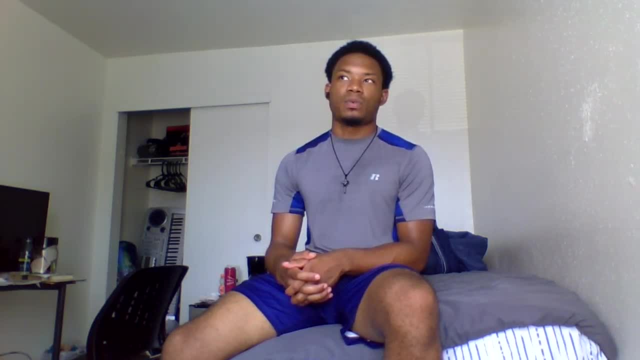 as music educators. you know we have to, we have to, we have to make a difference. so in your classes, you know not, don't just learn for you, learn for them, learn for that difference. all right, you may suck at spelling chords. i am not good at that. you may suck at spelling chords, that's okay. you fight. 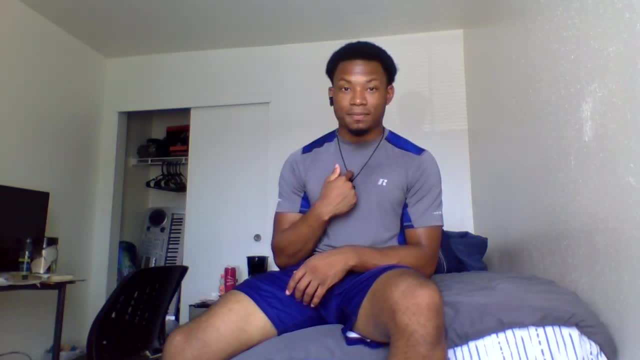 for it. do not let anyone change your mind, do not even let yourself change your mind. all right, this is not just for you, this is for them, this is for our future. all right, is it going to be hard? yes, life is not easy. all right, this is for them as well as for you, okay, um? 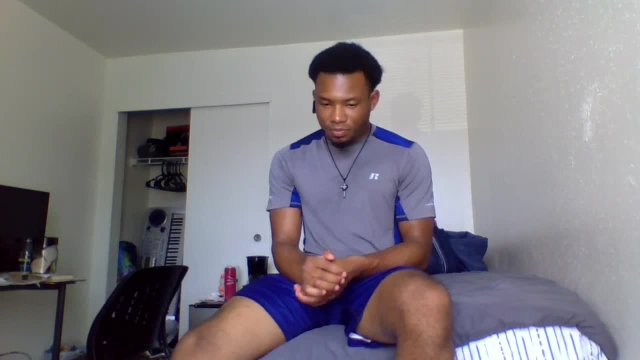 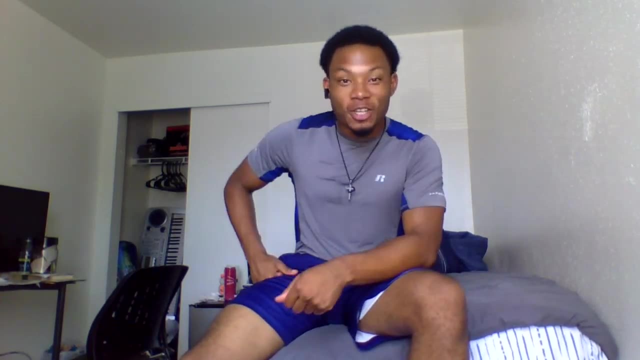 another thing also that comes with music education is like your core classes. you're good at that. you have all your classes finished your senior year. don't worry about it. okay, great pushers, you don't. you can clip out of classes your freshman year of college and be. 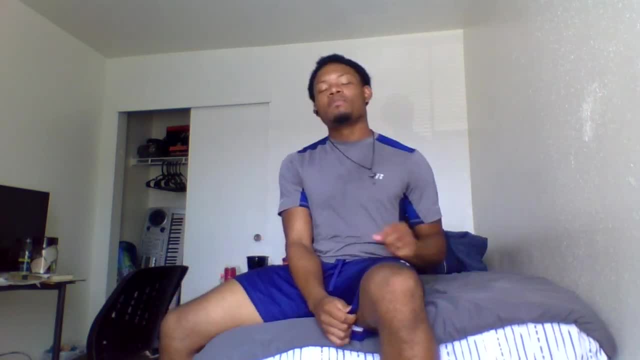 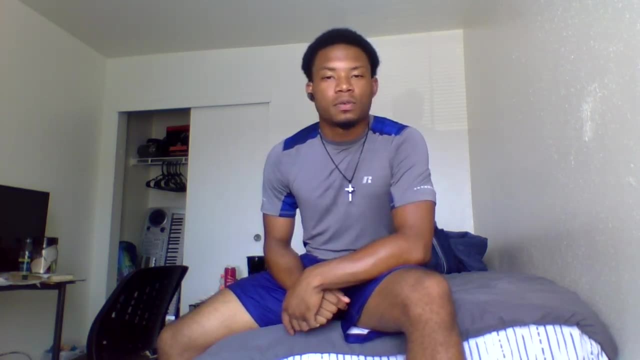 halfway, basically finished, but um, but yeah, that's your core classes, that's basically the life, um, also for all of any of you who are out there and you are, um, this is your senior year in a high school. the another another peek into my life as a music education major is we have to go to councils. 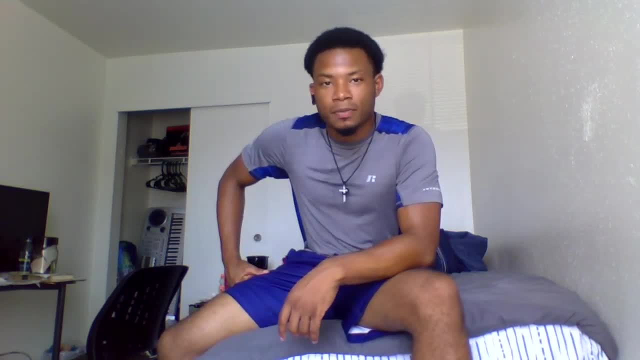 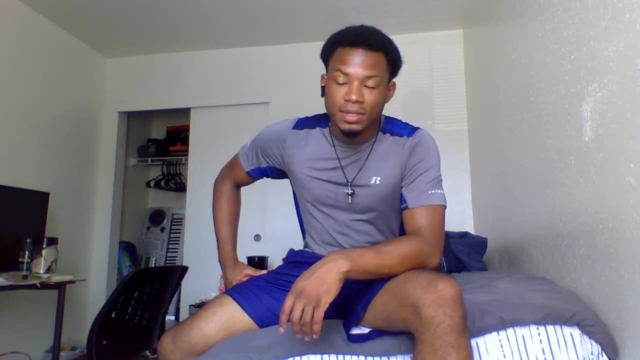 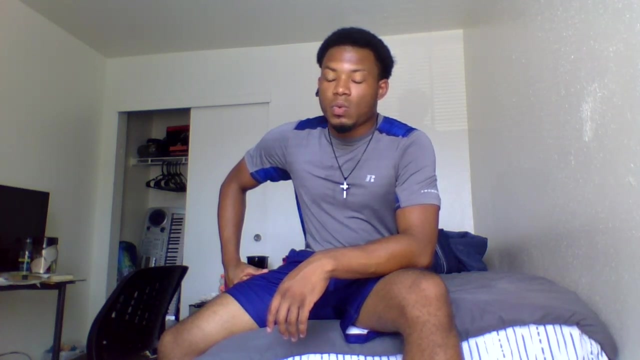 the same thing practically, but, yeah, you have to go to those. um, i, for one, i'm a student of northwestern state university, uh, of louisiana, and uh, one of the awesome things here is we, uh, we have a great staff, we have an awesome staff and they're very, they're very bright and, you know, they're very helpful. 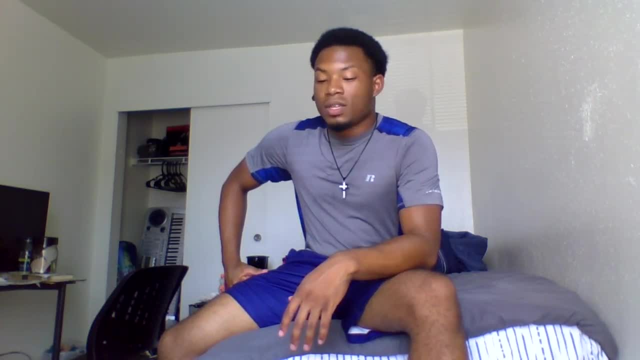 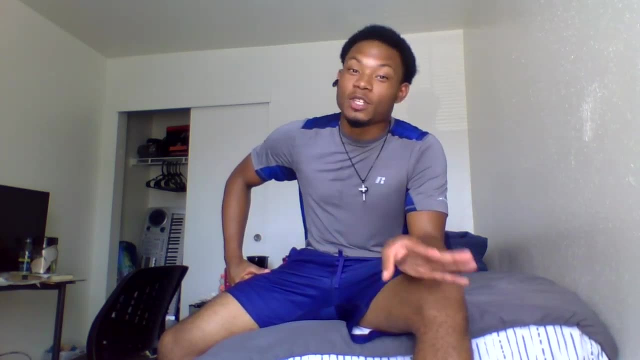 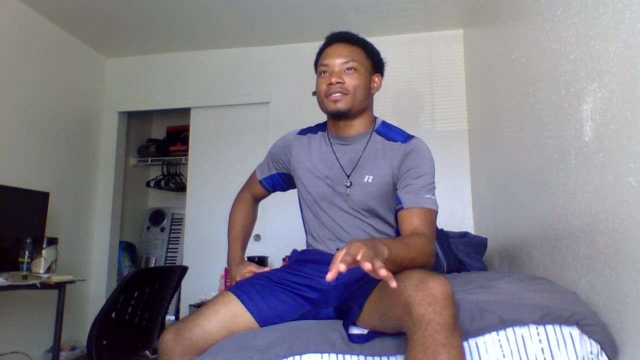 and um, well, i'm not, i'm just gonna be honest, y'all they're. they're ridiculously awesome, they're good, like our faculty here is like the music department and the music it's just crazy. it's it's crazy awesome, it's just awesome. my flute professor, she's too cool, like she plays awesome. 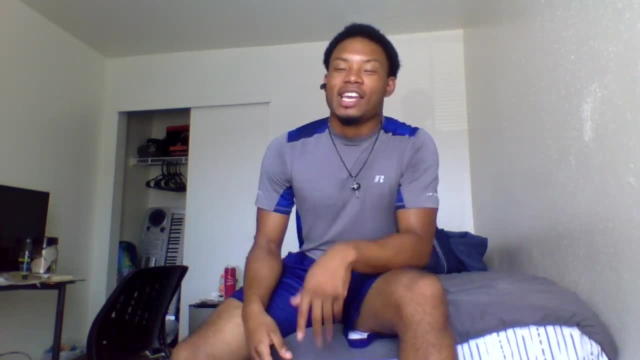 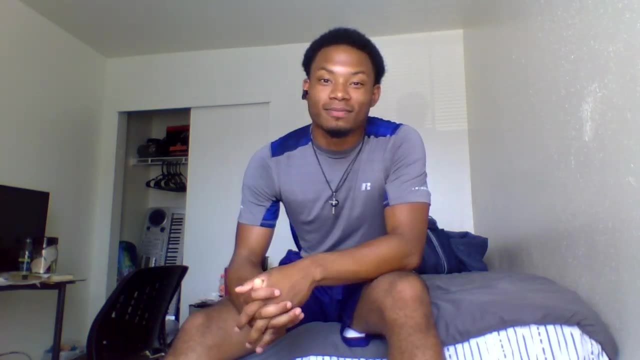 like it's just. it's hard even to say they're just awesome and like the university life. um, it's awesome too. it's great. i'm gonna cut him off. continue to use the word awesome because I like my university. I do, but the music world here is. 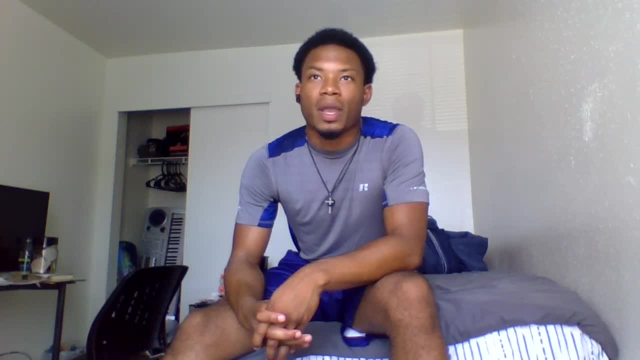 great and it's full of awesome and great leadership and faculty and you learn so much. you learn so much. you learn ridiculously so much you know about music and how it affects the world that you live in and how you can use it to help others. that's like the big picture. 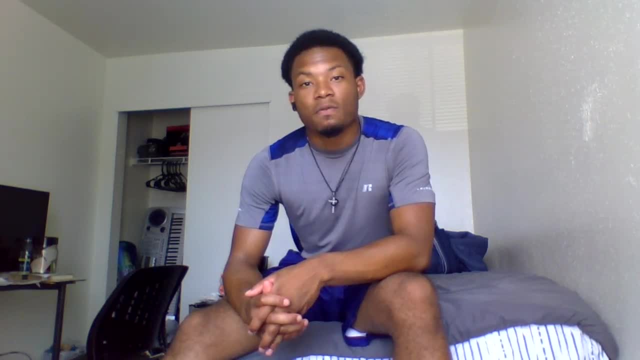 you know, as music educators, future music educators, how can we help others, how can we still live our lives but yet use music in a positive way in a world that is totally opposite? and that's just. that's basically our goals as music- future music educators. 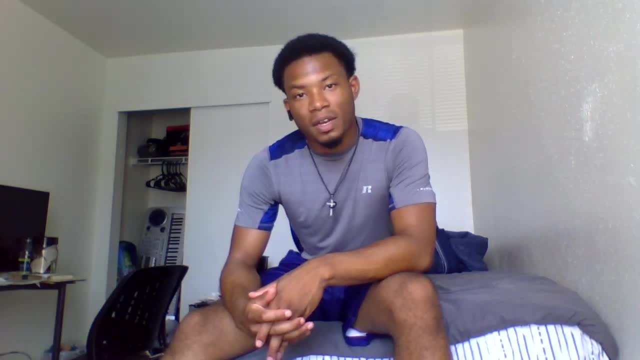 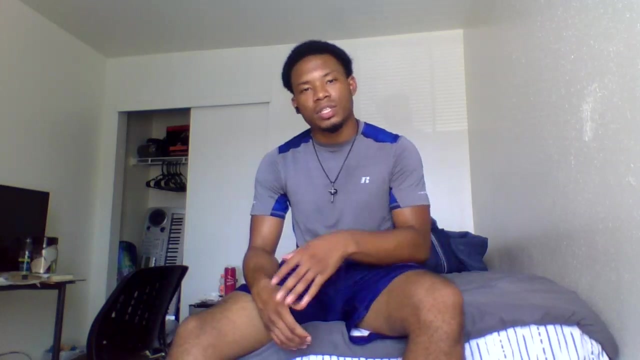 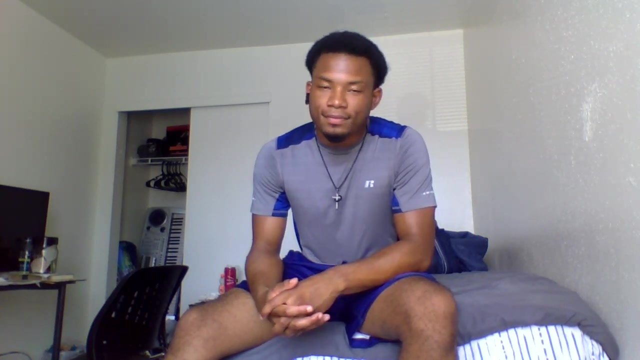 is to learn how to teach, be that motivator and basically break limits. you know, but I just still I want to encourage all my music educators out there. I want to, you know, let y'all know that. okay, I have struggles, we all have struggles. 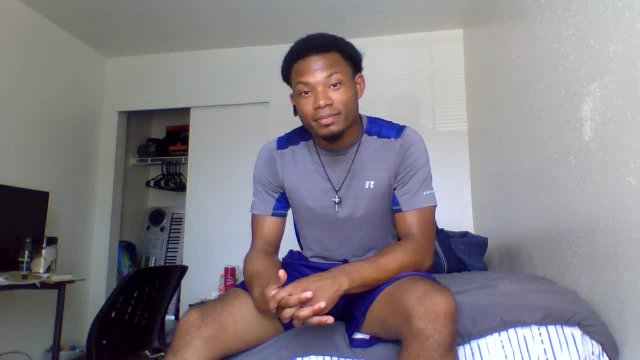 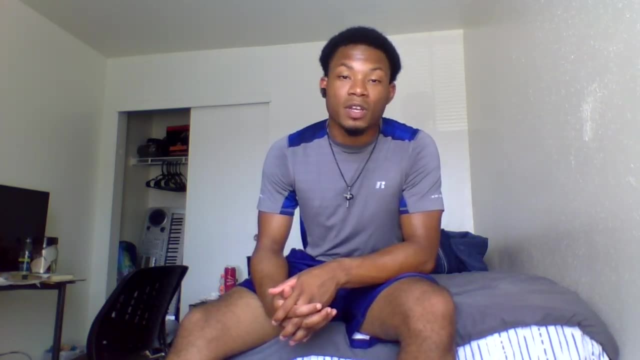 it's all great, we're all going to get through this. and you know, if you have issues in theory, if you have issues in R scales and piano, find somebody that's good at it, become friends with them. all right, I'm not saying. 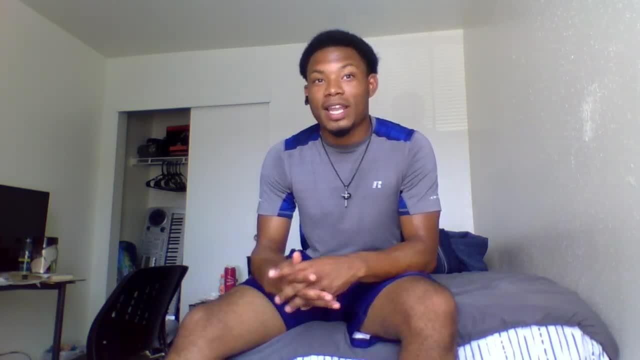 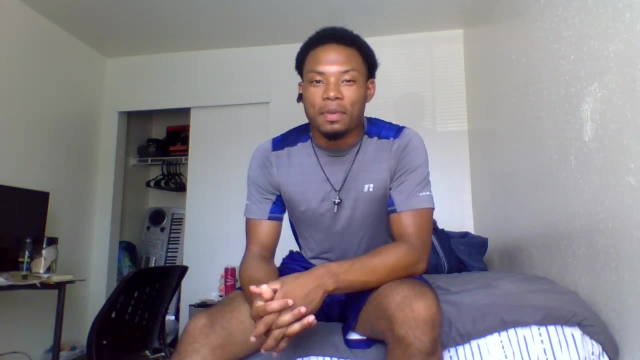 you're going to become friends with them. because that's just how we are music people. we latch on to each other like siblings and I have, like many of them in my section, all my piccolo people, like they're all my sisters and my brothers also. 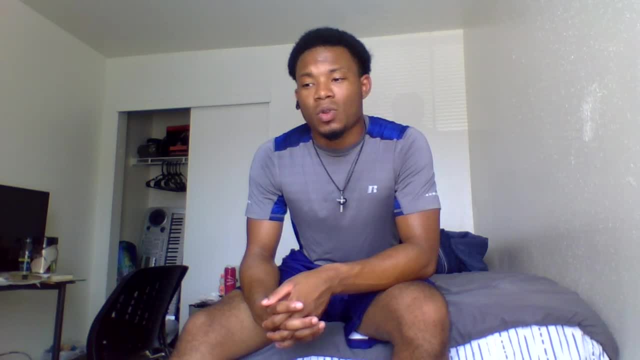 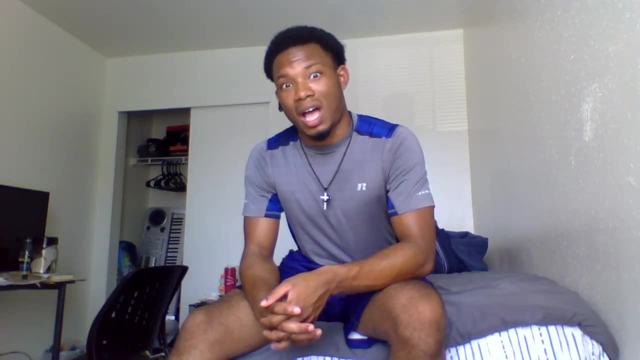 but find somebody you know who's good at those things and you know learn and ask questions and stuff, you know. don't think you're the only one that's struggling with this. there's many people and you'll come across a lot I've come across, so 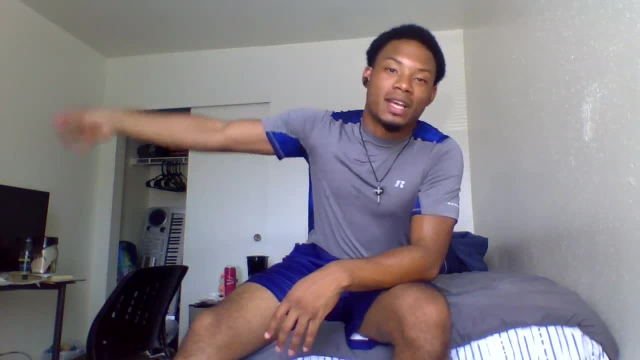 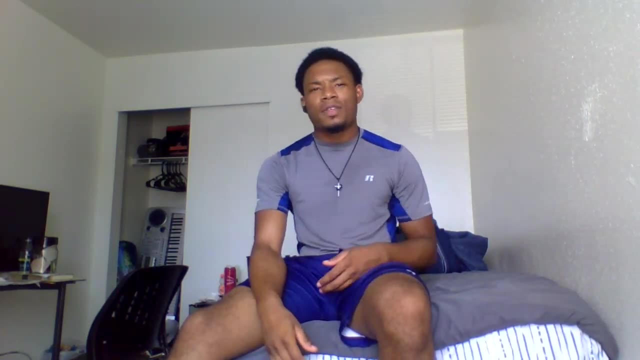 many people who basically have their bachelor's, who have their master's, who have their doctor's degree, who basically play in the military band or whatever, and they're like: well, I was bad at theory, but I got through it. I was bad at oral skills, but I got through it. 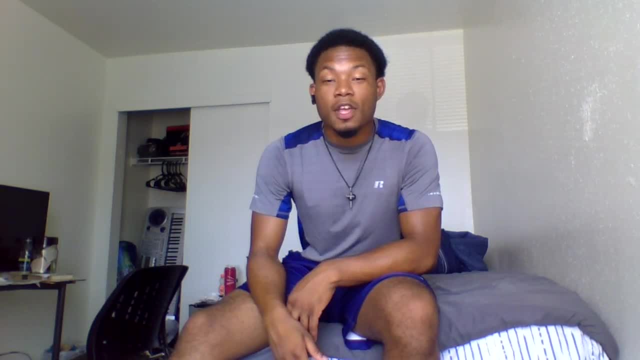 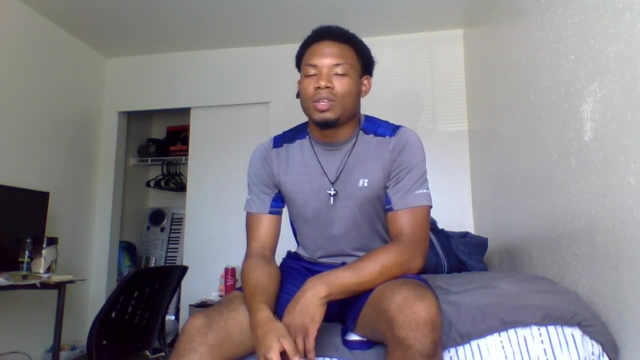 I was bad at music history but I got through it. I was horrible at piano, but now I'm playing this Bach concerto Or organ and whatever, and you'll see, you will never be the, you'll never be the first. 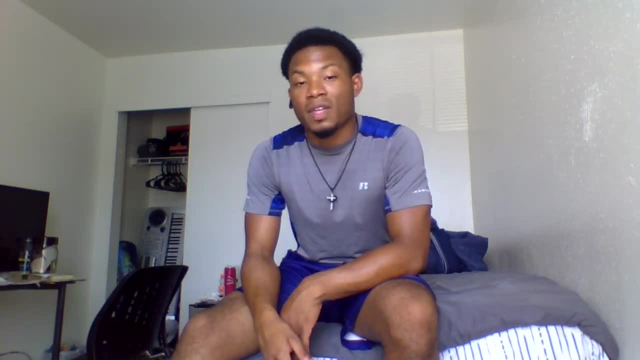 you'll never be the last. there's always someone out there that is doing this, that's having the same trouble as you are, and don't think that this stuff is not for you. if you love music, you continue to pursue, to pursue music. you push yourself even more and know that. 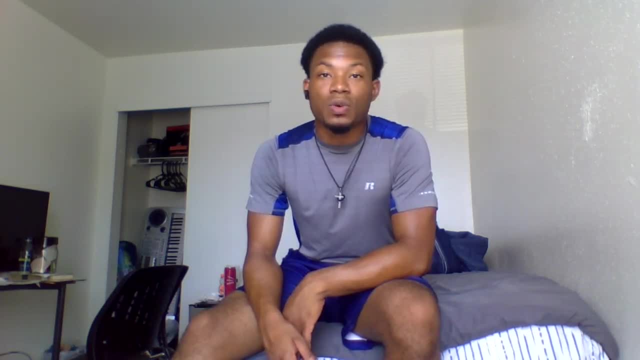 don't just do it for yourself, do it for the children, do it for our future, do it for the future of America. the difference is not just small, this is a big difference. so if you have struggles, if you have doubts or whatever, get rid of those doubts, don't worry. I myself 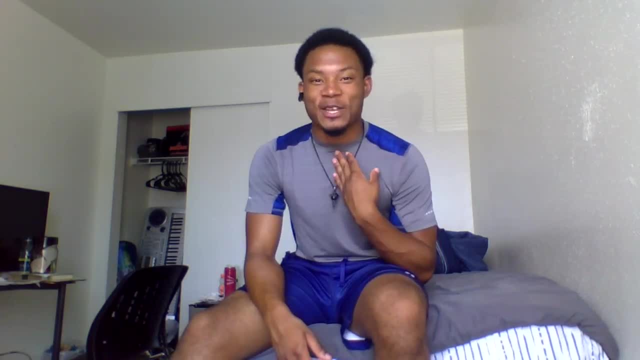 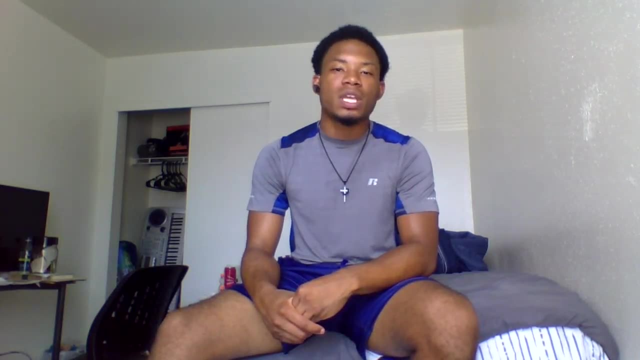 I doubt a lot. I do, I do. but the reason why I'm telling everyone else, you know: because I know that we can do better. I know that we're capable to do better and by us knowing that we can, we can push ourselves even further more to want it even more. 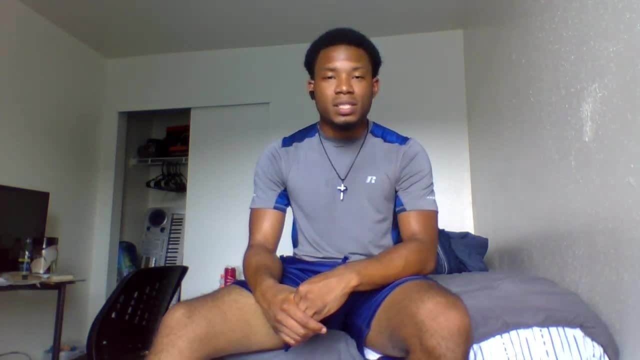 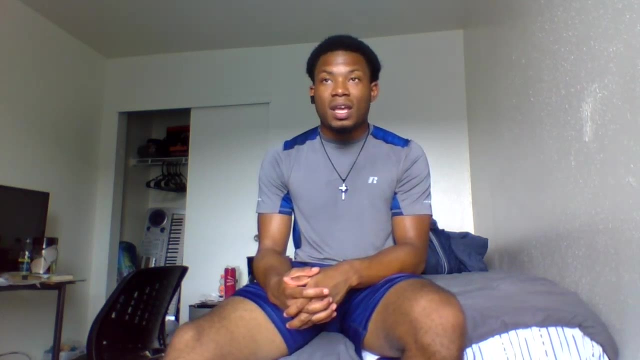 and y'all it's powerful, it's, it's this is a thinking kind of thing. y'all this is a mentality it really is. you have to really think and you, you have to think of this as, like you know. 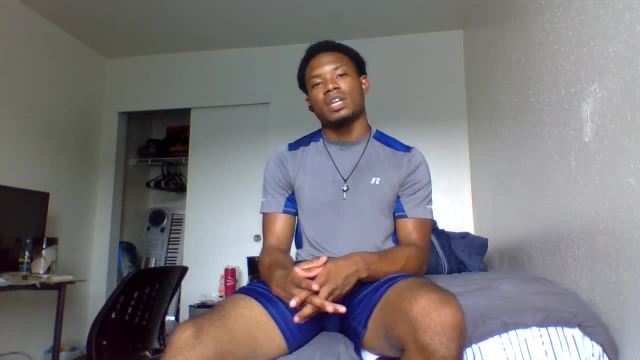 this is what I want for my life. this is something I want. this is something I want to make a difference in. if I have to work hard at it now, then I will. I don't know, I don't, I don't. 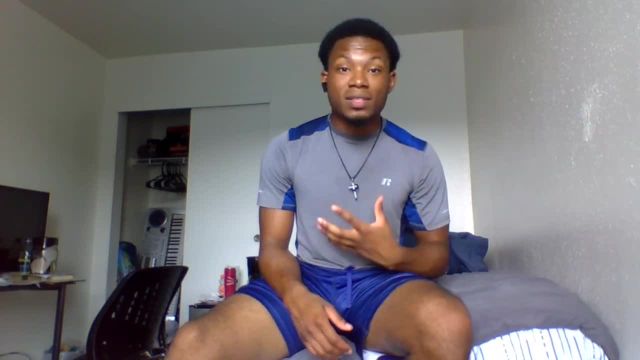 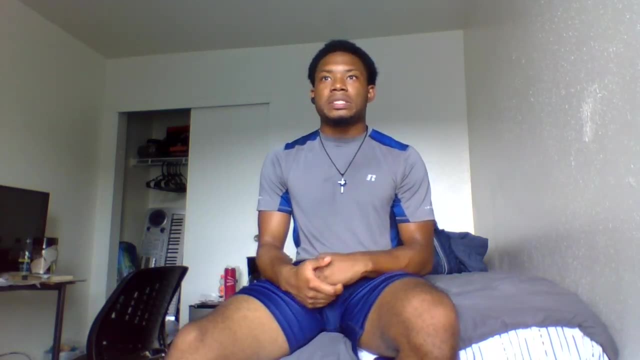 I don't care how long it takes. I'm going to get this, not just for me, but for those students out there, those kids out there, those, that child who is who, who's, who's having a hard time at. 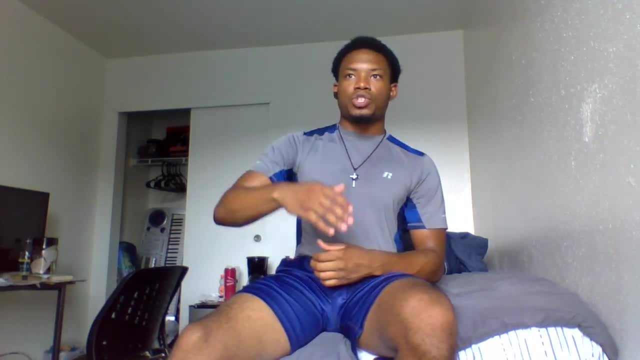 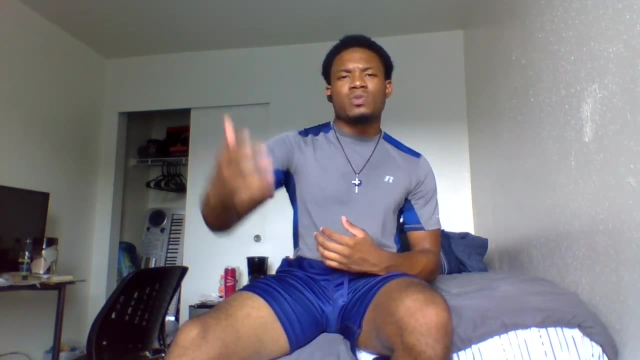 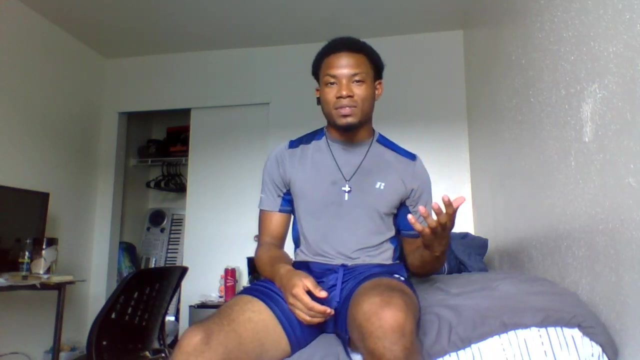 home. I want to be able to be able to show him, you know what all that anger and all that rage that you have. I can show you how to use that and produce a great sound into an instrument, how you can basically give them a gift that they can use for the rest of their lives. 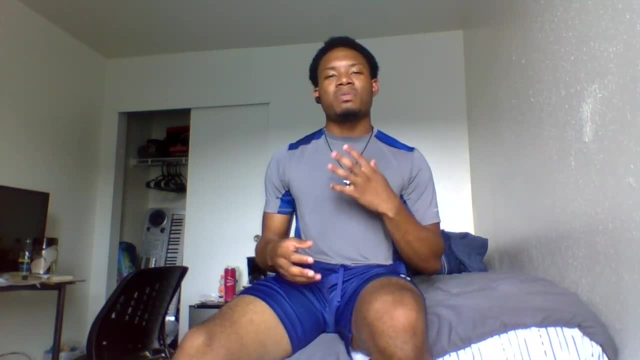 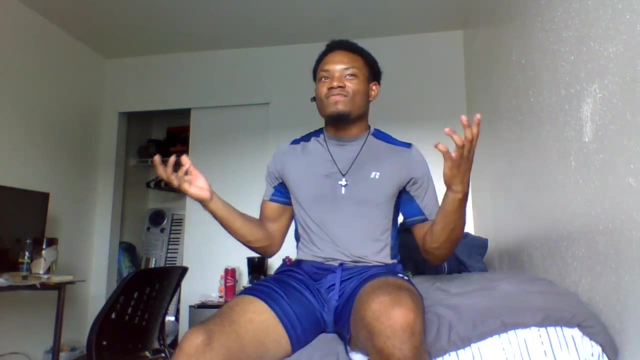 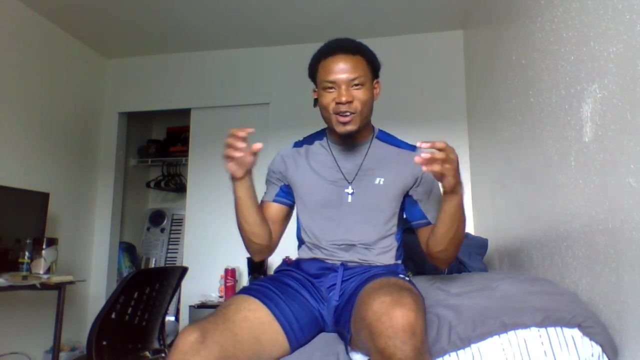 no matter what they're going through, they can pick up an instrument and be able to play and be able to express how they feel through that instrument. Y'all. it's like, you know, if everyone was musicians and we would all live in a very perfect, you know, perfectionist kind of. 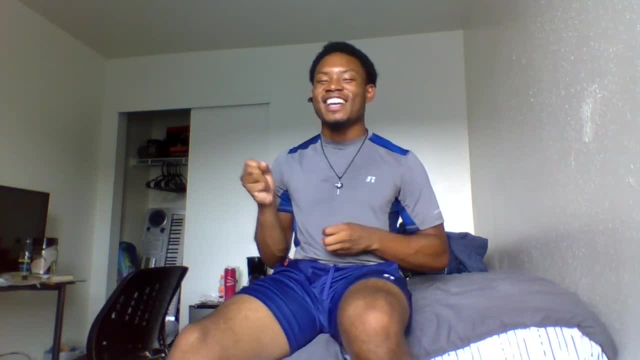 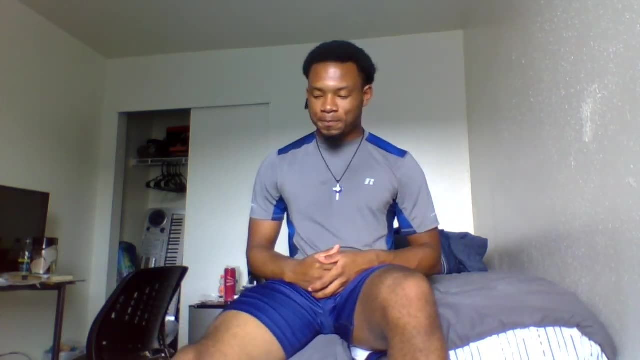 you know society, because every musician is a perfectionist. no, you know it's. it's a whole bunch of you, it's a whole bunch of you. so, but you know, I've understood that, as musicians, you know we're hard on ourselves. 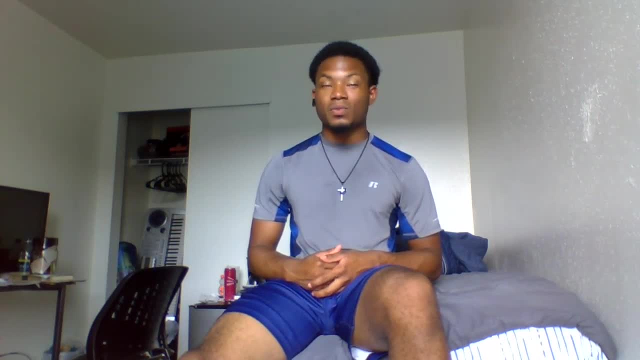 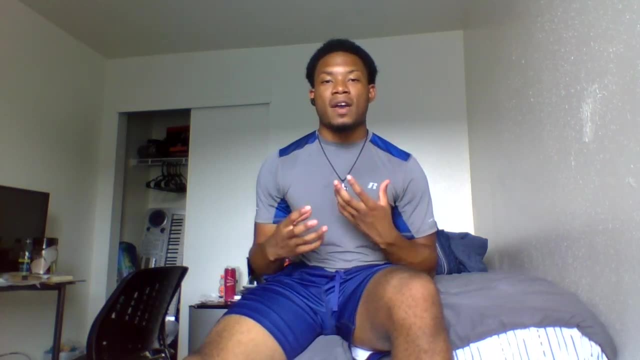 Some of us are hard just to be hard on ourselves. Others we're hard on ourselves because we want more, we want to understand more, we want to do more. We realize that the more we have, the more we can do, the more we can use, and I personally see it as like this: 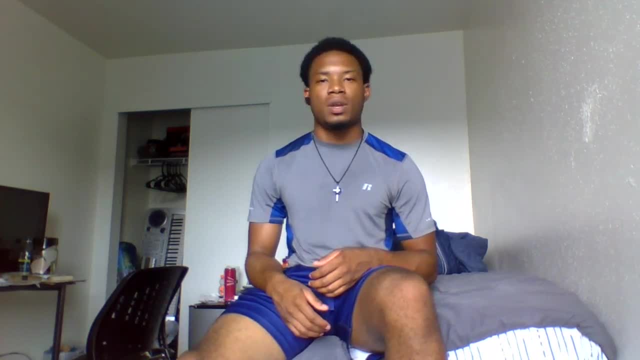 All of my struggles and everything that I struggled with, whether it be theory or oral skills or whatever. I've been through a lot of things and I've been through a lot of things. Sometimes those are, those are all skills. 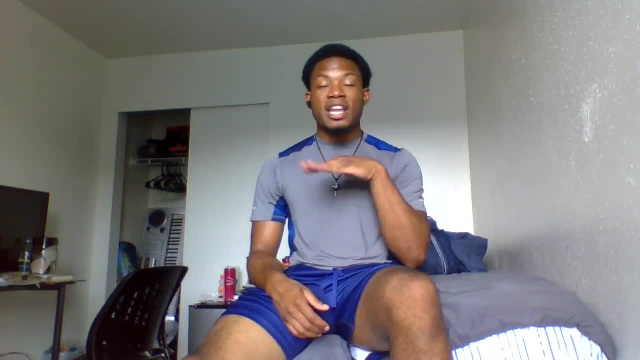 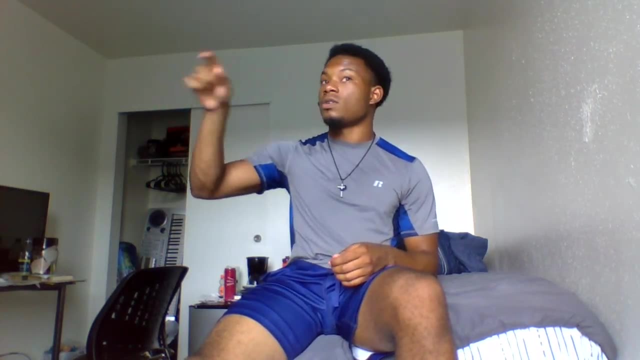 Some of you who are coming from high school may not have developed those skills. You got to come across people who have developed them And they're like stupid, awesome at them, like they're fahk, I mean, they kill it. 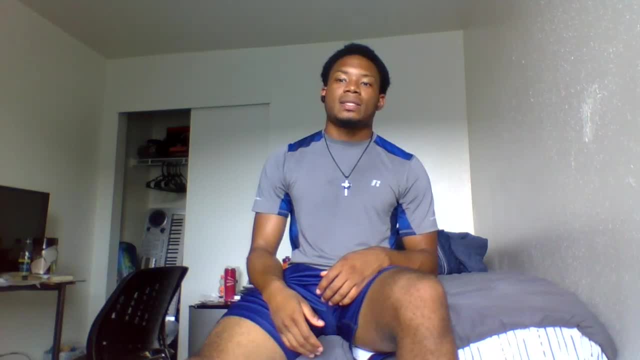 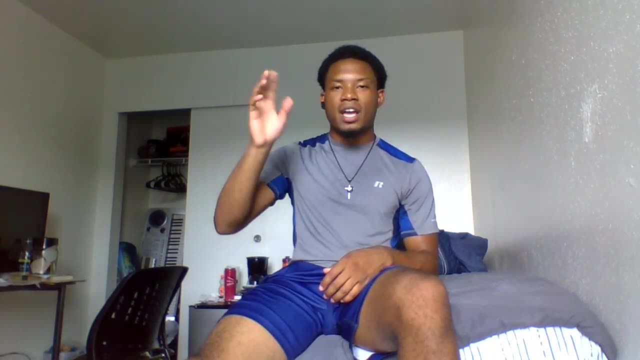 And I see that as like: okay, that's fine, It's cool, But if I'm having issues, you know, going from dough to me, you know—that's fine, that's cool, That's great, It's all great. 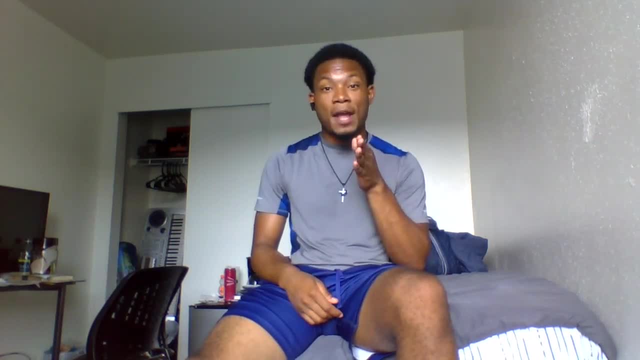 Some of you are like: no, that's not great. No, it is great. You know why? Because I'm putting forth effort and I'm trying my hardest, No matter how long I'm going to get it, I'm going to get it. 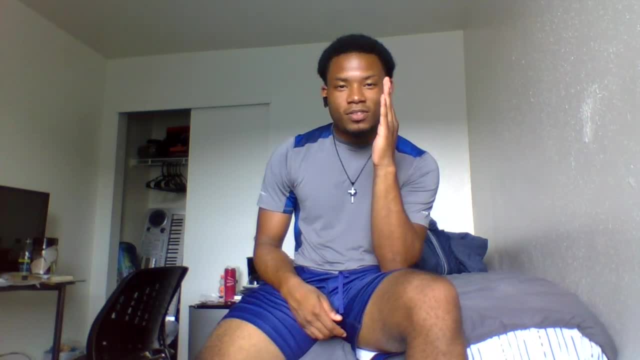 So I want to encourage, strongly, strongly encourage y'all, because this is not just for y'all, This is for me also. I'm going to encourage every one of you who are born in music. Y'all, this is the greatest major ever. 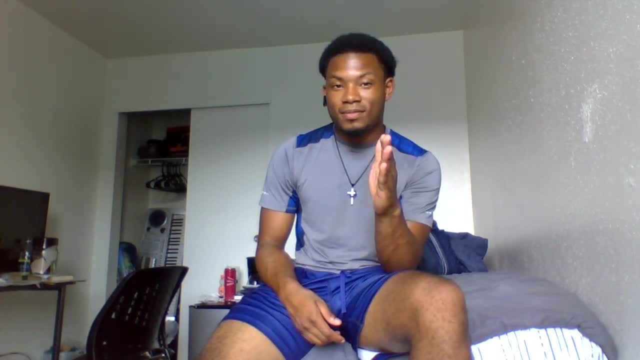 It's not the easiest, It's not the hardest, All right, But you can make a great difference, not just for you, before our future. So go into this happy and excited, because you're going to learn some awesome stuff And there's so much to learn. 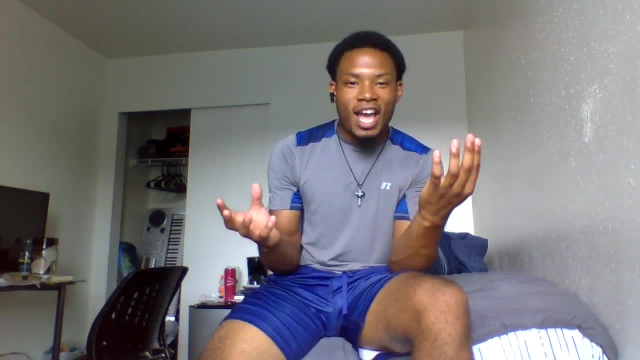 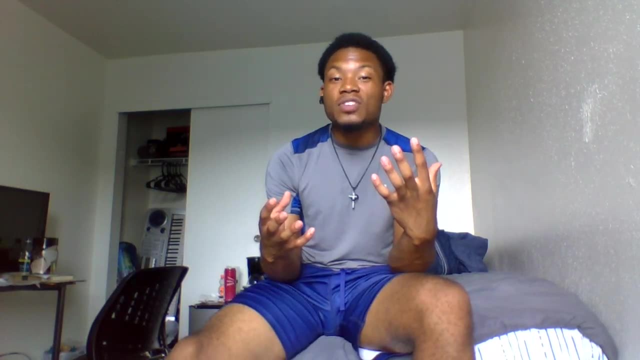 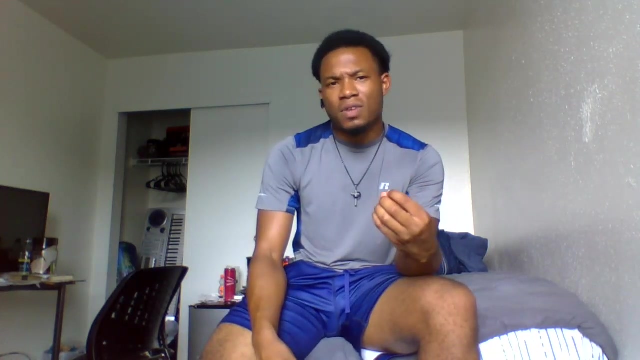 And it's so. it's crazy how the music world is And you'll hear some of the most beautifulest music. How many beautifulest, Beautifulest, The greatest music. You'll learn how to express yourself in the music world. 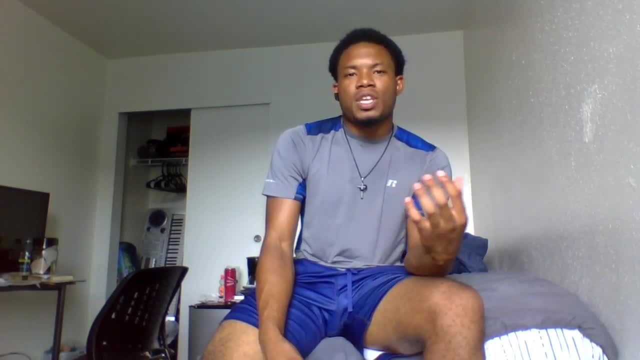 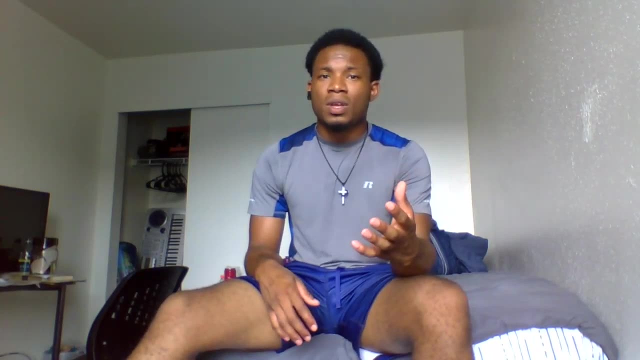 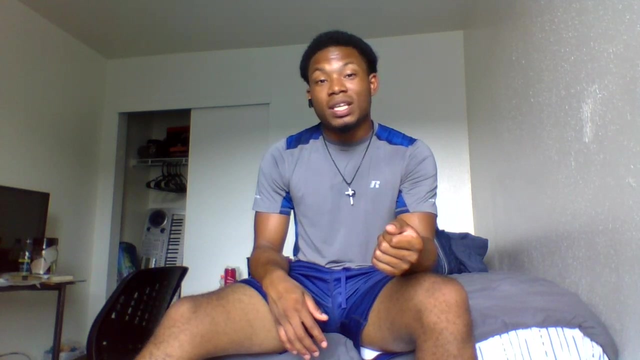 And you can compare yourself from three years before now and you'll see how fast you grow. you know, under great management, under good faculty. You know, And it's a great experience, It is, It's life-changing, It really is y'all.